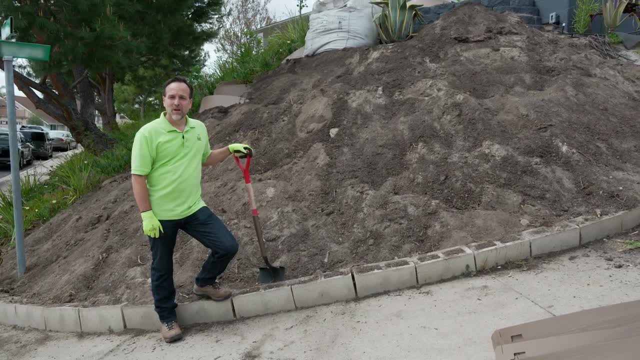 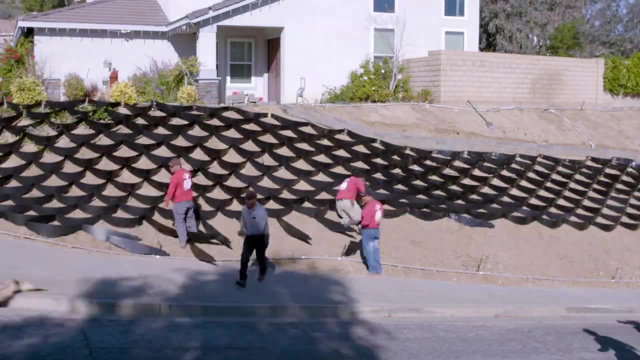 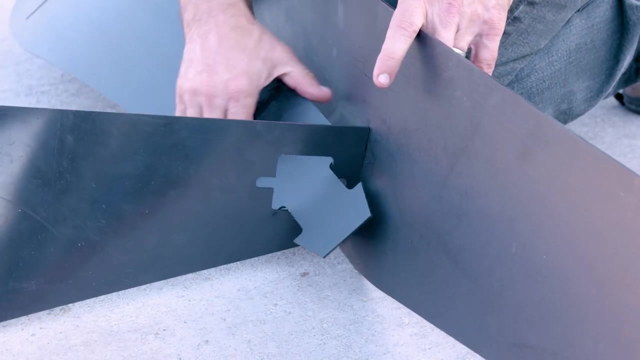 Hi, this is Mark. We're here in Mission Viejo, California. We're going to do an installation of the Dirt Locker. The Dirt Locker is a product made of 100% recycled plastic, made and manufactured in the United States. It is used to address hills exactly such as this, to create a beautiful 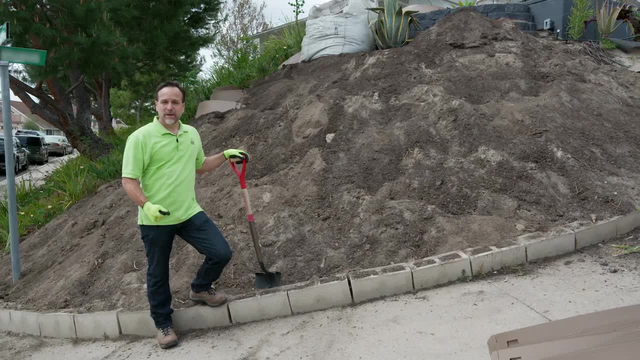 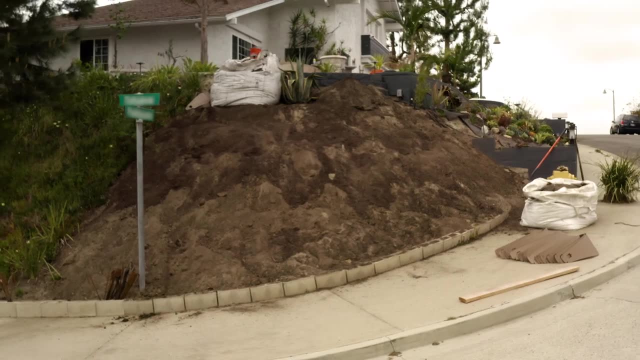 garden where it was once very difficult to grow things. In this case it's even a little bit more challenging because it's on a corner. So today we're going to talk with the homeowners of this corner lot and find out why they chose the Dirt Locker system to resolve their problems. 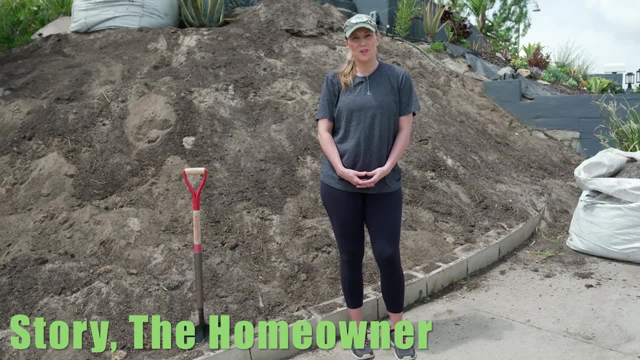 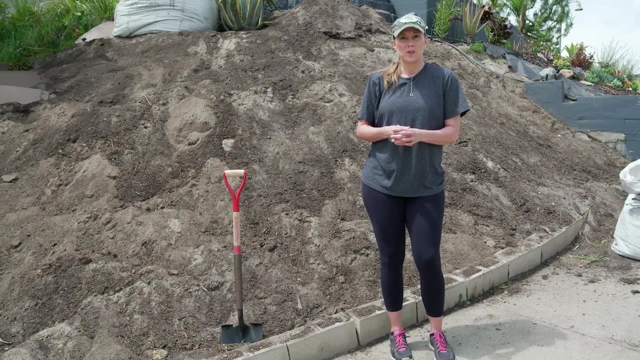 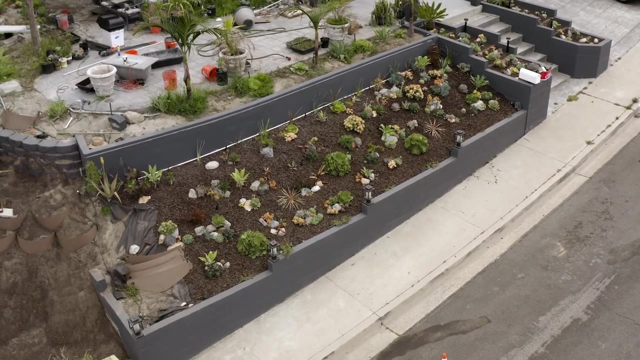 and reduce cost. Hi, my name is Story. I live in Mission, Viejo, and the majority of our house is wrapped in a hillside. My fiancé did all of the labor in actually putting in a retaining wall in a portion of the hillside and it was not only very costly but the labor 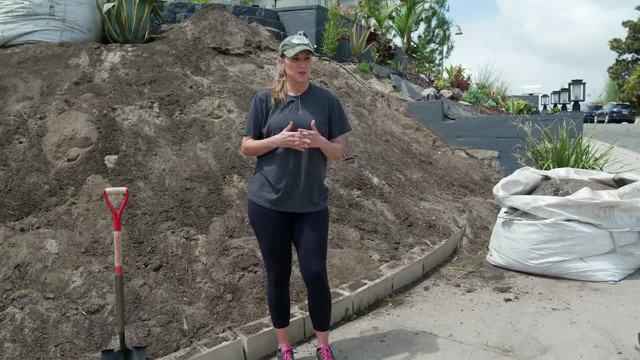 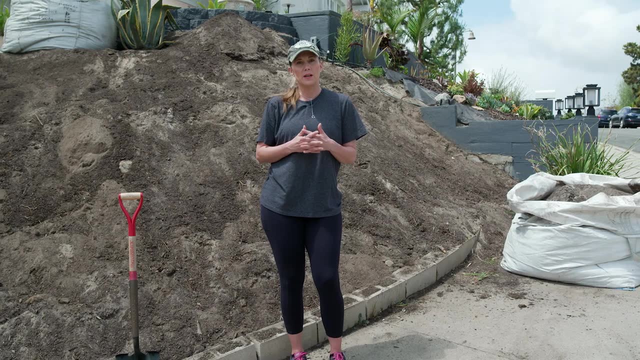 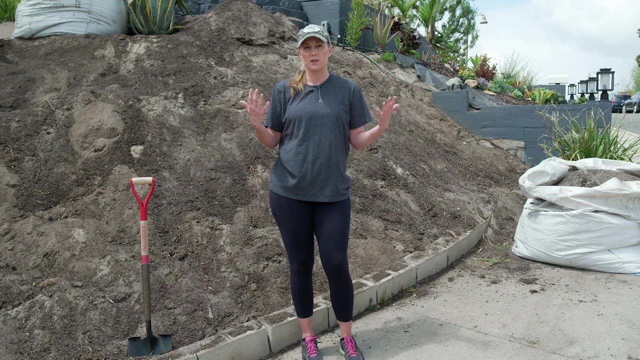 that he had to put into it was a lot, So I thought there's got to be other options out there other than building a retaining wall. So one night I googled hillside landscaping and the Dirt Locker videos popped up and I watched every single one of the videos and I was instantly sold. They solved. 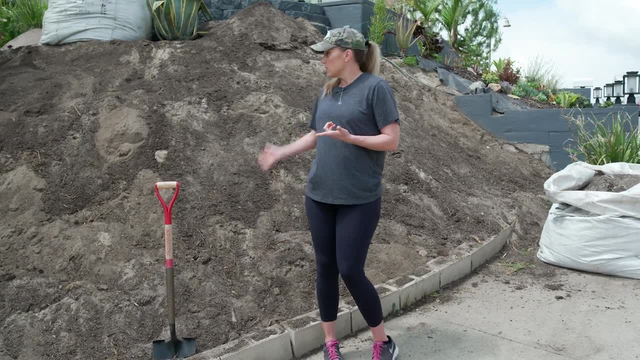 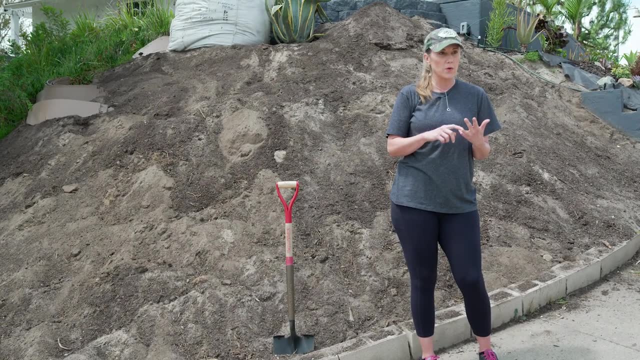 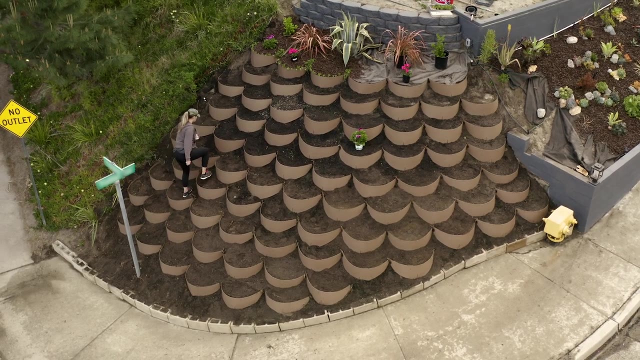 all of our problems. It was the erosion problem as far as the dirt, retention of water for the plants and then also something that the retention walls didn't give, was an option to walk up and have steps to maintain. You're still going to have weeds, no matter if you put down weed guard or you're going. 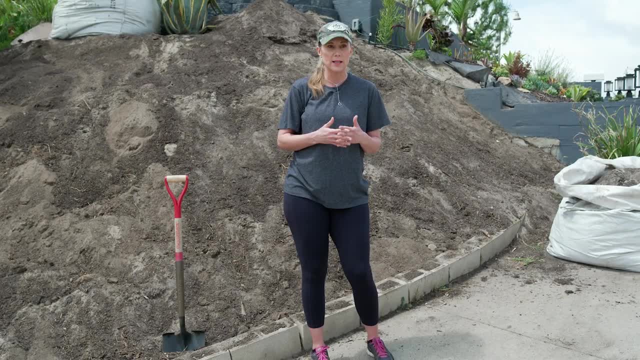 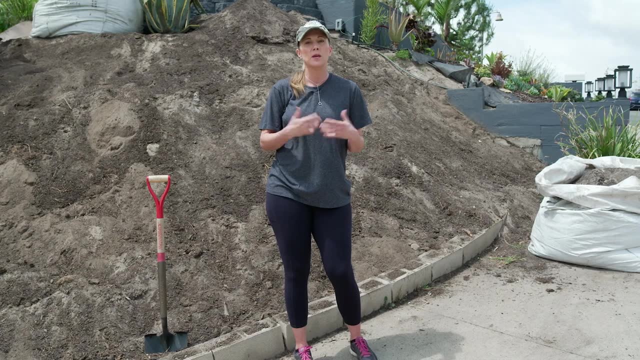 to have overgrowth that you need to maintain, so you need to access those plants, And the Dirt Locker did all of that, and it also seemed to be made out of a material that would last a very long time. So if you're going to put forth the effort and the money, that was important to me also. 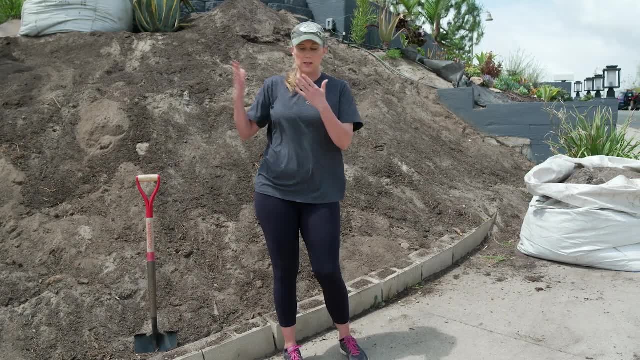 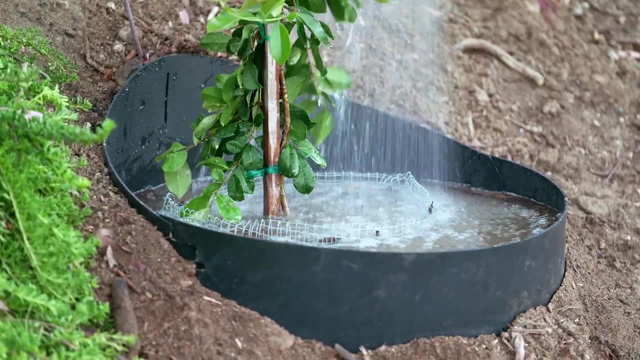 And not only could you have a Dionne and a lower- iniciativeness project, but it was also important for the you do the hillside landscaping aspect. if you had a single tree, like a fruit tree, that you wanted to put on the hillside, there were also options for that to help retain the water and the root system. 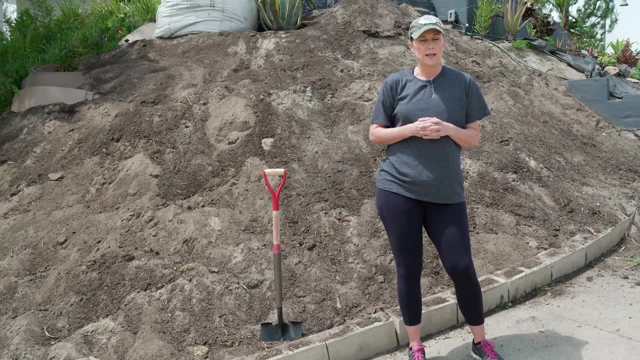 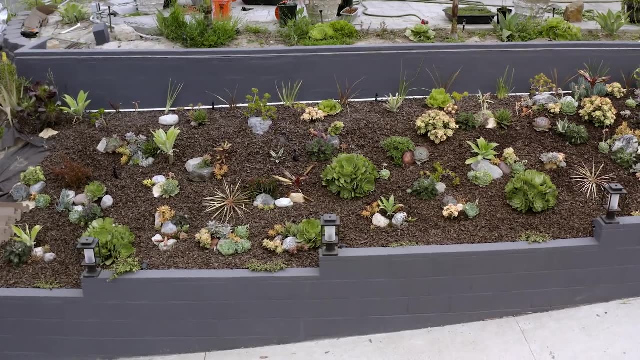 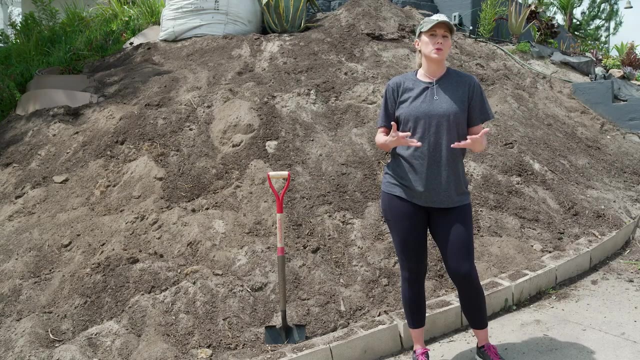 it seemed very simple, it seemed logical and a lot easier than a retaining wall and aesthetically the retaining wall is very harsh in my eyes. it's very status quo in most of the houses and the dirt locker gives you something aesthetically that you can't do with a retaining wall. staggering the 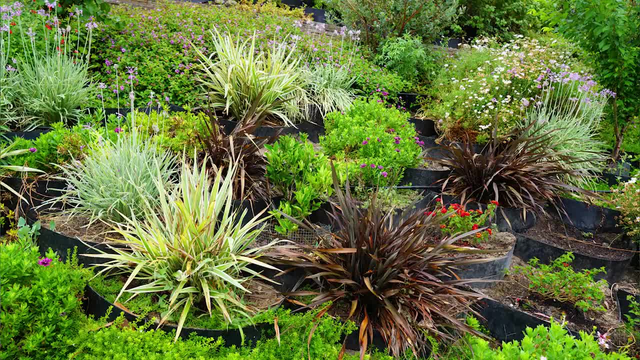 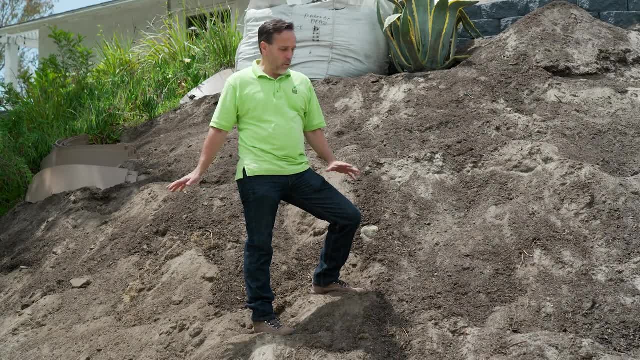 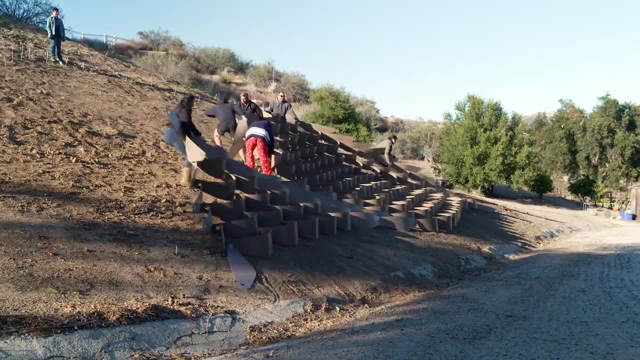 plants and having the growth fall like a waterfall. so those were the things that interested me. the key difference between doing a dirt locker system on the on a corner hillside versus a flat hillside is that on a flat hillside we would assemble the dirt locker network on the ground. 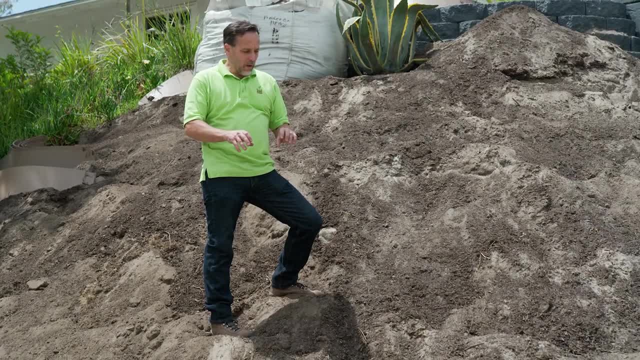 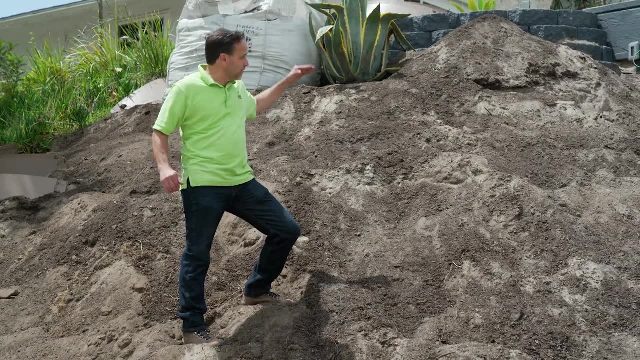 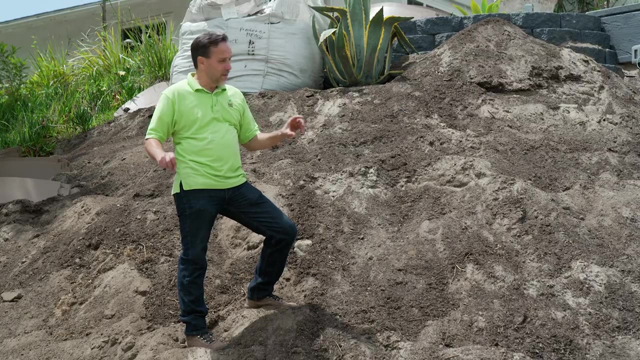 and pull it up as a single unit. well, on a corner that doesn't work the same way because of the changing length as you go from the top of the hillside to the bottom. So each row has to be created individually, and that's what we're going. 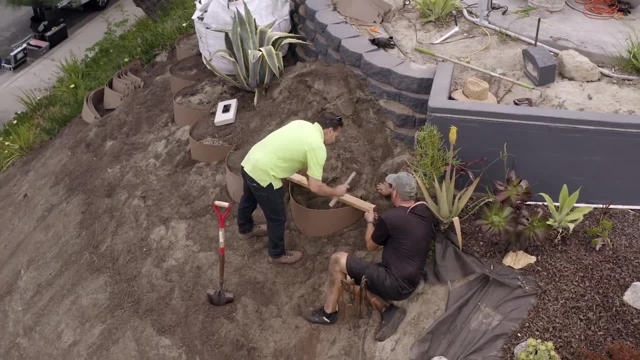 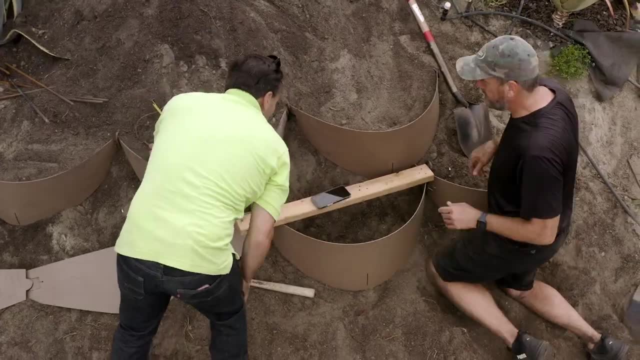 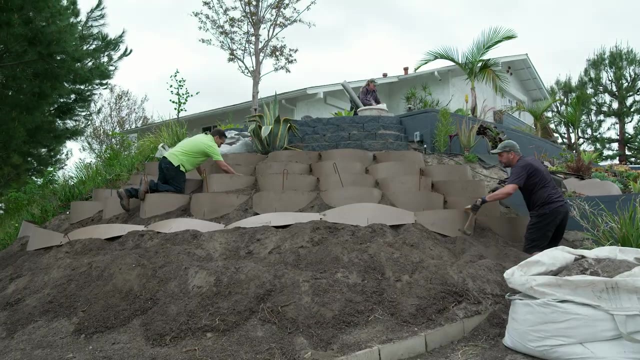 to do. Starting at the top, we install our first row. All the dirt lockers in a row will be connected to each other and staked down. Each dirt locker row will be independent of the other rows. Using a phone app as our level and a two by four, we make sure that each dirt locker is level from left. 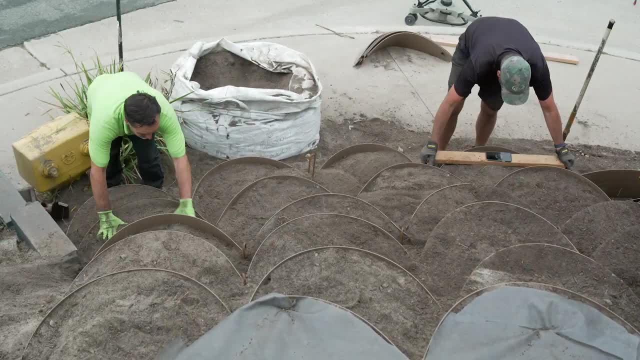 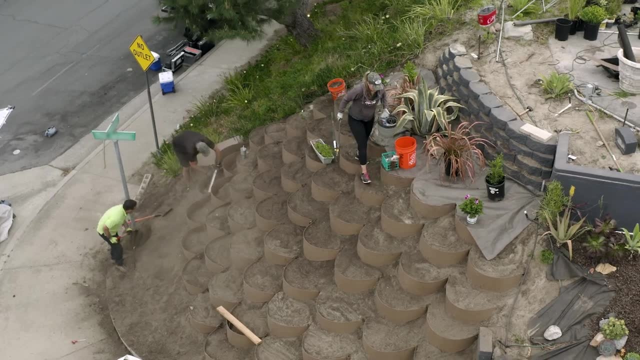 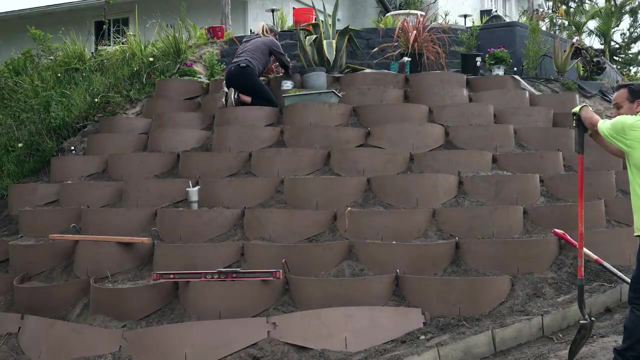 to right and from front to back. We make sure that all dirt lockers in a row are positioned in a straight line. Notice we are using backfill to help us position, shape and secure each dirt locker. Each individual row will be customized to fit the contour of the slope's rounded shape. We're still 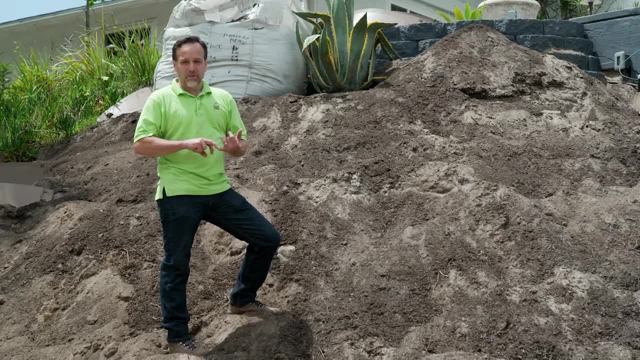 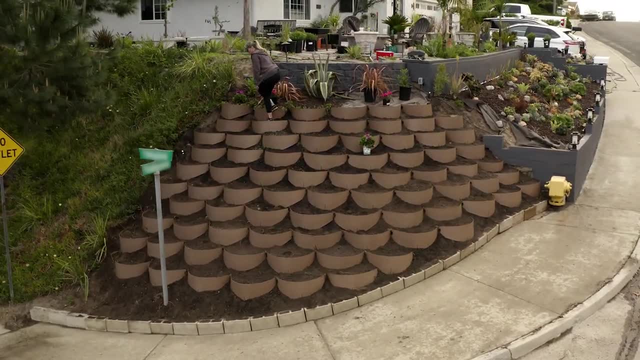 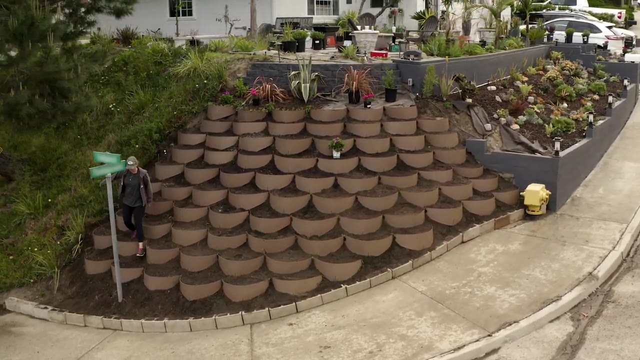 going to have the same dirt locker capabilities in terms of being able to traverse the hillside. We're still going to have the same water retention capabilities. Everything about the product itself in and how it's helpful on the slope remains the same. It's just the installation that 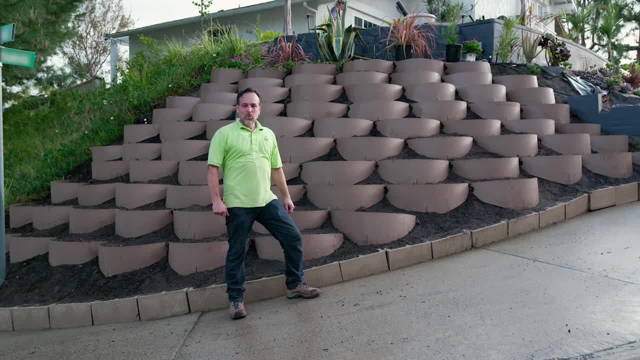 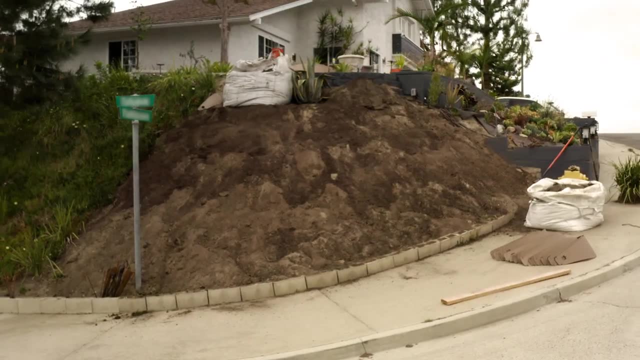 differs a little bit. So today we were able to install 78 dirt lockers. The homeowners started with a steep eroding slope on a corner lot that was unsafe to work on and unable to sustain plants. In less than six hours we transferred the dirt locker to the hillside We were able to install. 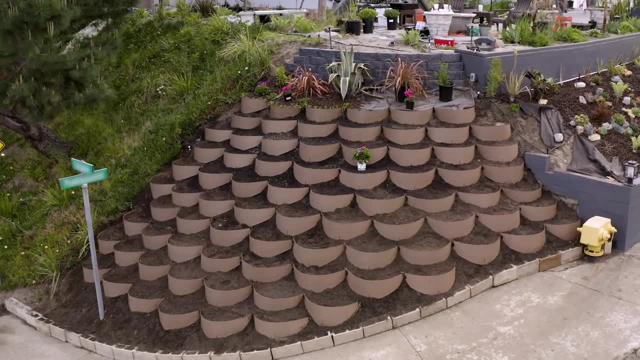 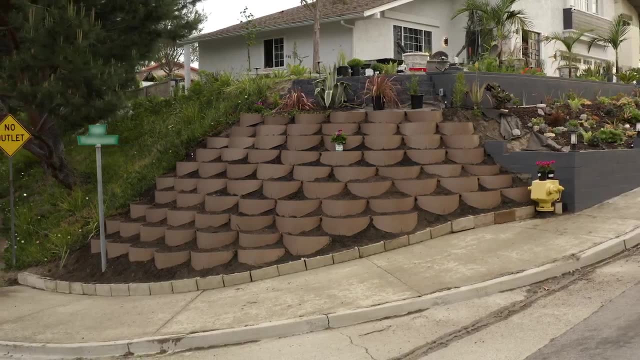 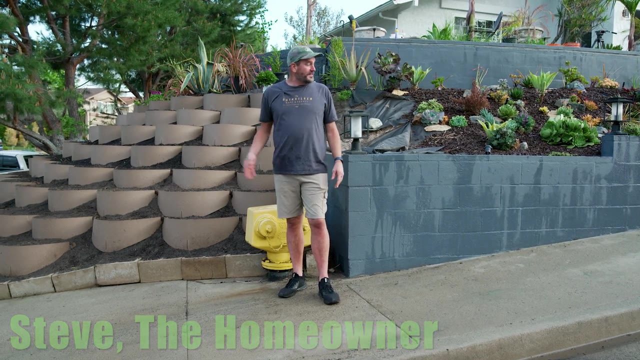 78 dirt lockers and transform this problematic slope into a beautifully terraced hillside that is now safe to access, ready for planting and soon to be an amazing garden that the homeowners can be proud of. Well, after spending a day working on the dirt lockers, comparatively to the retaining wall that 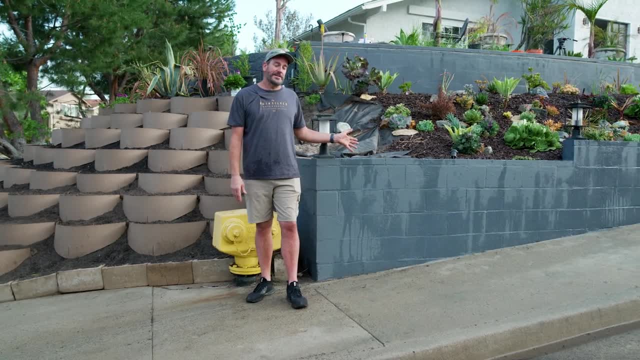 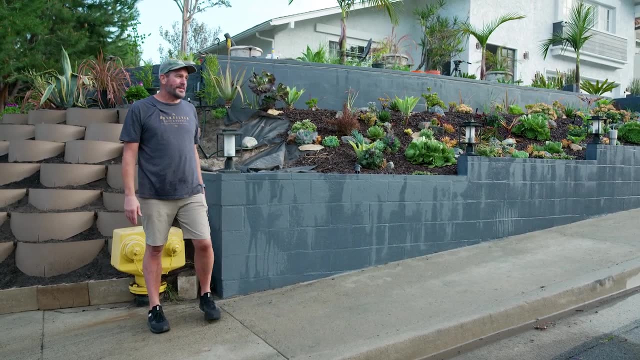 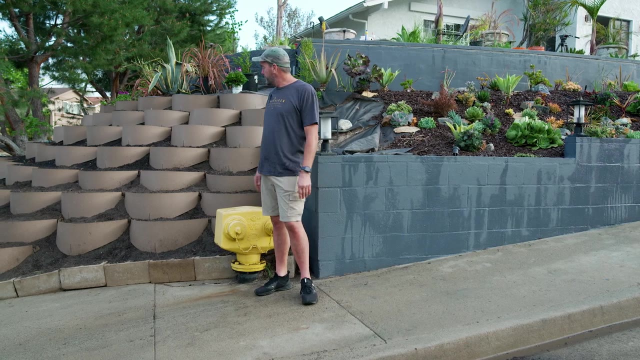 I built. this took about four and a half months of my time, Pretty much every weekend, and I think a little bit of my soul's in it, that wall. but this we did in about five and a half to six hours with two of us, so it really 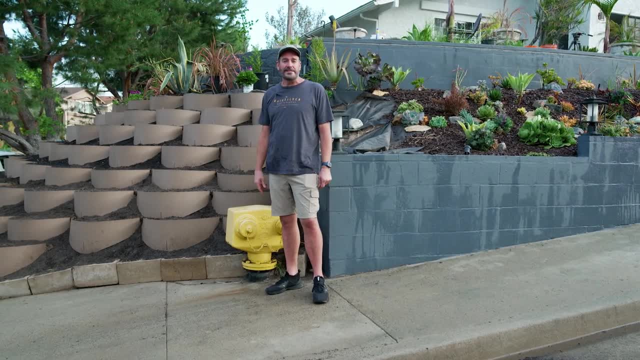 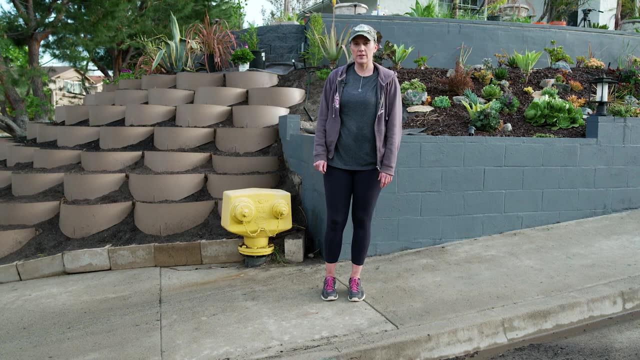 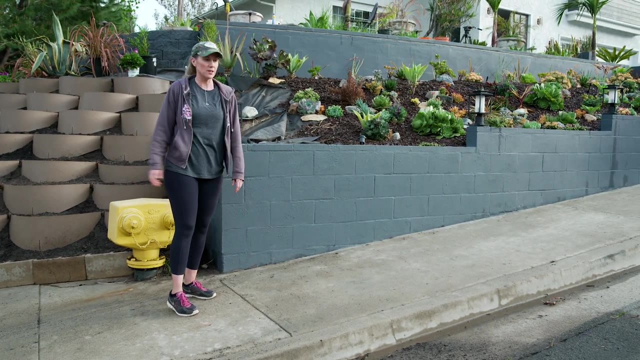 really made a difference and it looks beautiful and I can't wait to get the plants in because I think it really, really enhances the beauty of the of the corner. All right, I think Steve already covered the mass amount of labor that it did to do two retaining walls compared to doing the dirt. 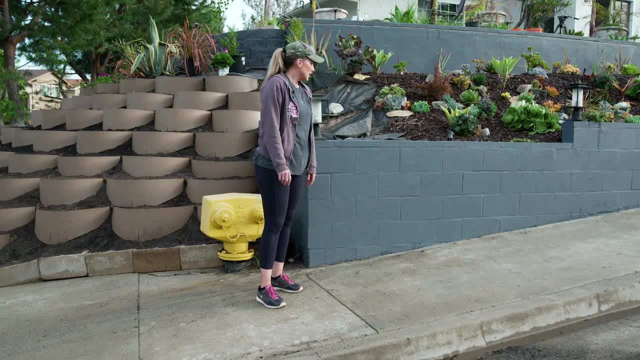 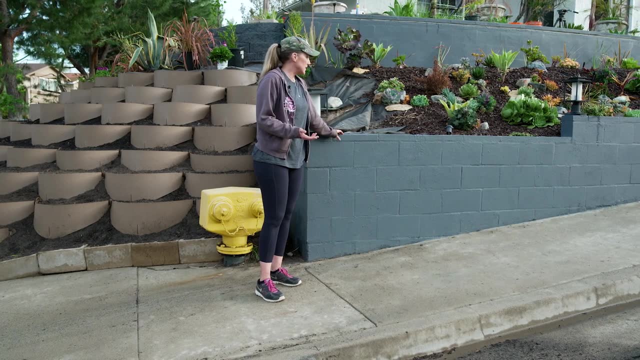 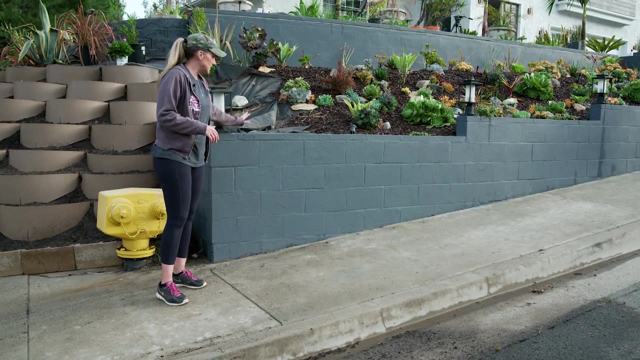 locker in half- more than half the time. but I want to talk to you about the aesthetics. A lot of the houses have retaining walls or they're just layering bricks. It's very harsh, as you can see. I do have plants that'll eventually drape over, but it's going to take a lot of plants to cover. 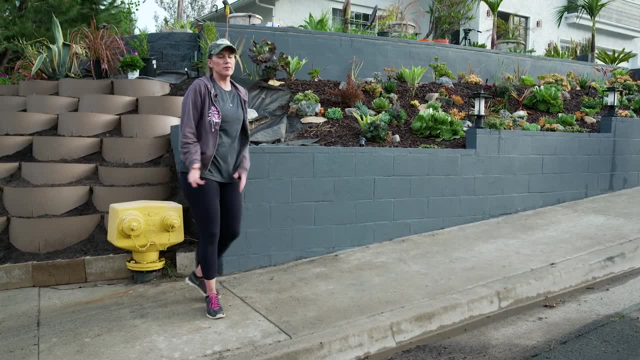 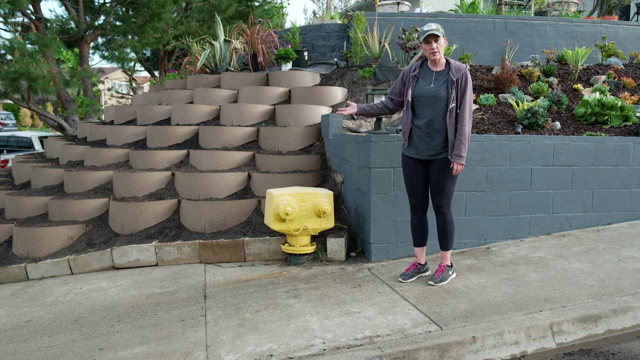 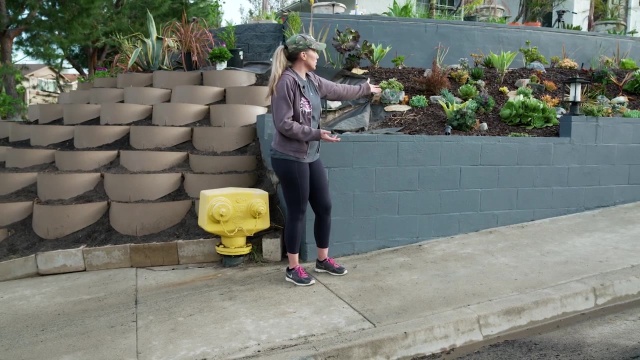 this harsh cement, whereas you have the dirt lockers over here, which give it much more of a cascading effect. Obviously, there aren't plants in here, but there are going to be. Another pro and con of the retaining wall is: I still have a slope, so water is still going to run down and if I need to step in between the plants, 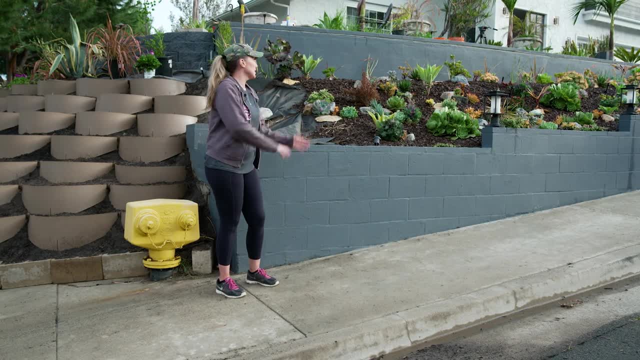 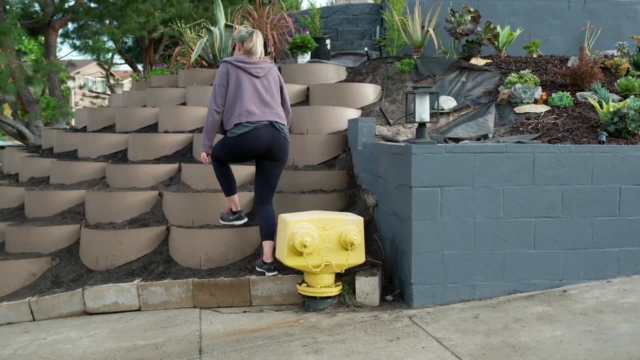 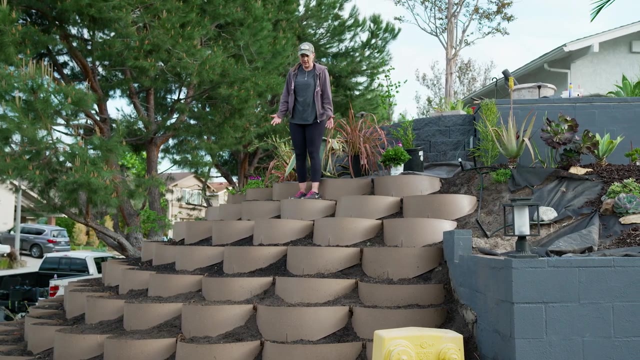 yes, I can, but all of my mulch is going to go down. I have to replace it or I have to crawl on my hands and knees. versus the dirt locker, I can easily and safely walk up and down. obviously, there aren't plants in here, but we will be making some throughout. that are steps, and 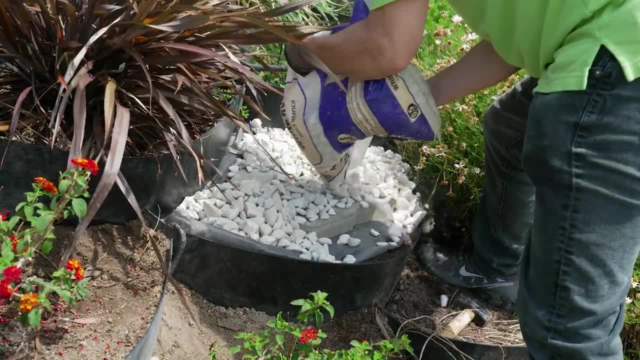 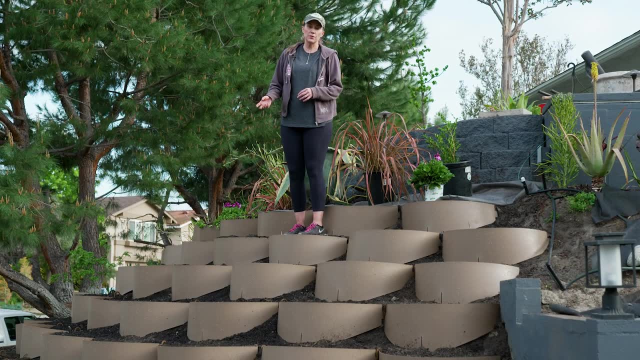 Mark's got a separate video on how to do that: devoting a whole dirt locker for a paving stone so that you can step in between, maintain your plants, whether that being pulling a few weeds here or there, want to change some plants, or you want to prune some plants back, and that's what. 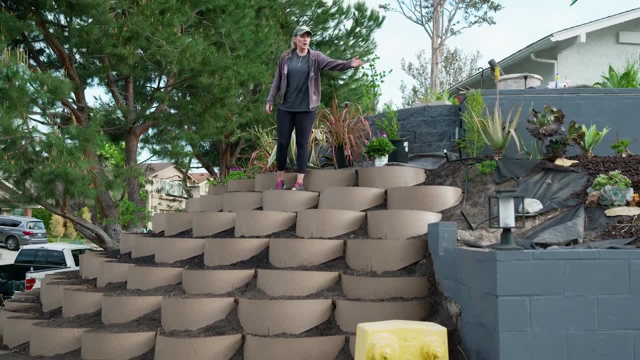 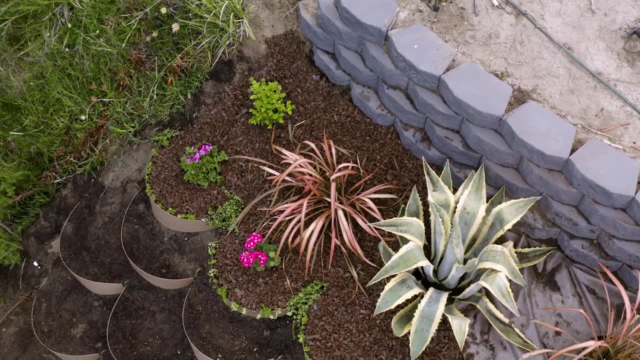 the great thing about the dirt locker. Also, it's going to take me a long time to drape that wall versus with the dirt locker. I already have some that are draping, that will drape from the top and the plants that I put in.